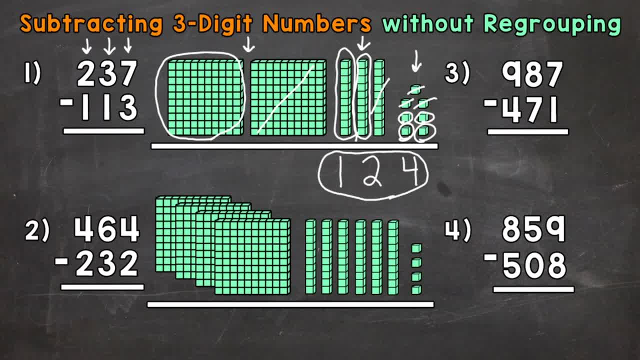 So our final answer: one hundred twenty-four. Let's solve this to the left. So we have one in the hundreds place. Let's solve this to the left, where we have the original problem as well. Start with the ones. So seven ones minus three ones gives us four. 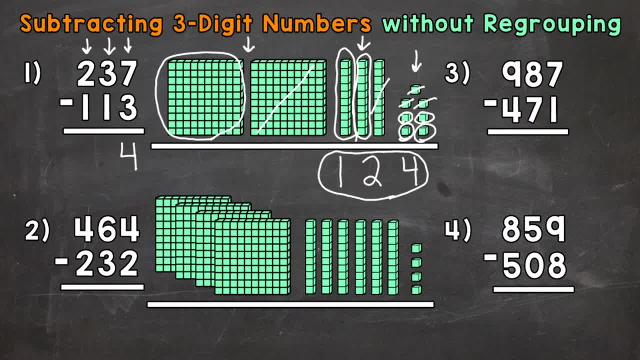 Move to the tens. So three tens minus one ten gives us a two in the tens. And then lastly the hundreds, So two hundreds minus one hundred gives us a one in the hundreds. So we get one hundred twenty-four. over to the left as well. 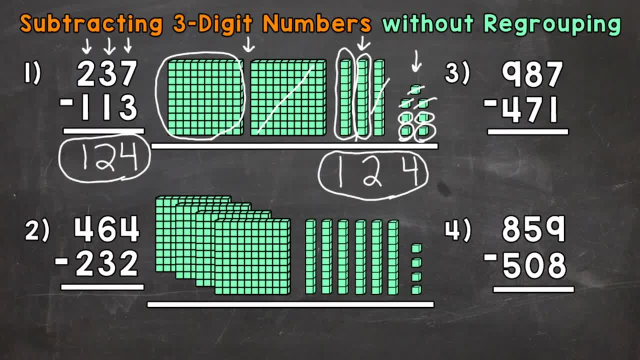 Let's try another one and move on to number two. So we have four hundred sixty-four minus two hundred thirty-two, So starting with four hundred sixty-four, And we are subtracting or taking away two hundred thirty-two, So we have four hundred sixty-four, represented by base ten blocks. 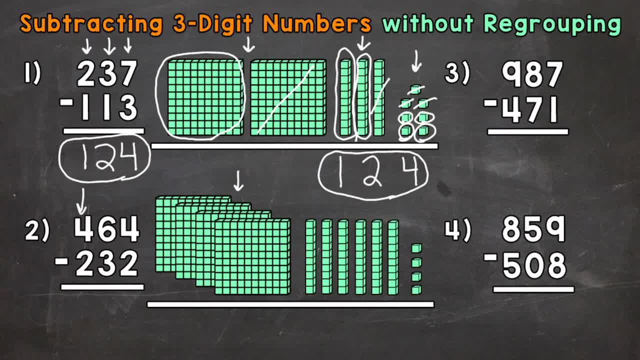 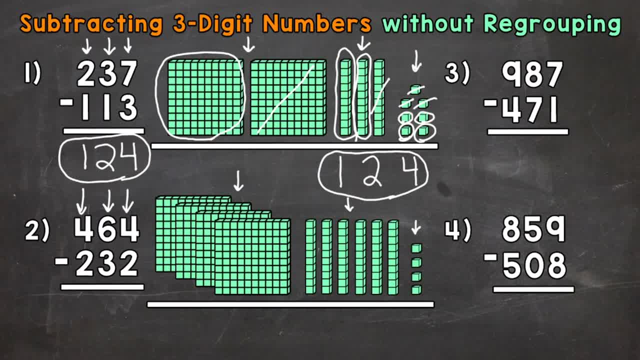 A ones in the hundreds place, We have four hundreds, And then a four. in the ones, We have four ones. So let's start with the ones, Four ones minus two ones. So let's subtract two ones, One, two, And then let's see how many we have left. One, two. 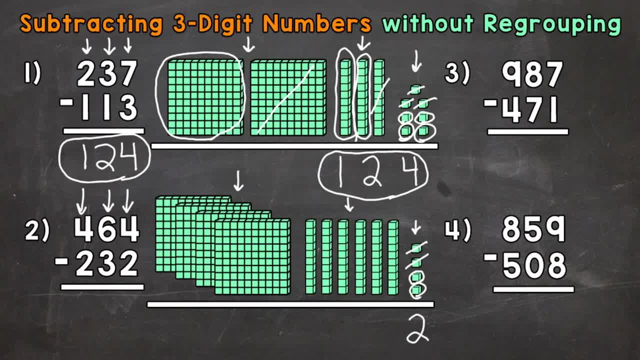 So we put a two in the ones place in our answer. Let's move to the tens place. So we have six tens minus three tens. So let's take away that one hundred twenty-two away. three tens, One, two, three. How many do we have left? One, two, three, So we put a three. 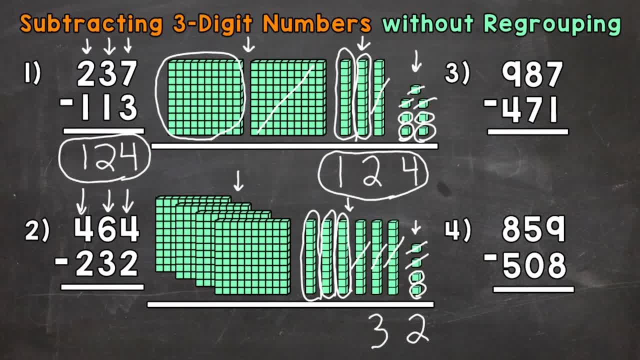 in the tens place in our answer. And lastly, we have the hundreds, So we have four hundreds minus two. So let's subtract or take away two, One, two. So how many do we have left? Well, one, two. So we put a, two in the hundreds place in our answer. Final answer: two hundred thirty-two.